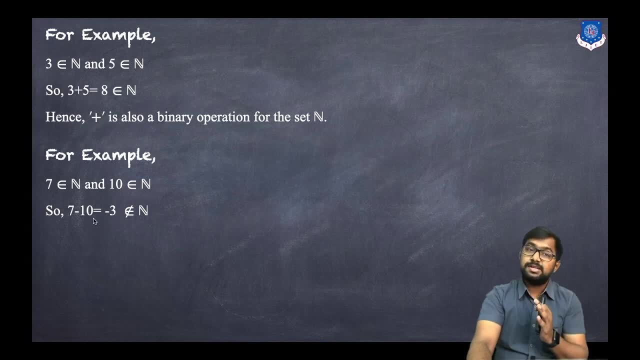 or if we use this minus, So 7 minus 10.. So that is negative of 3.. And we know that this minus 3 does not belong to set of natural numbers. So what we can conclude? so hence this negative sign. So hence this negative sign. it is not a binary operation. 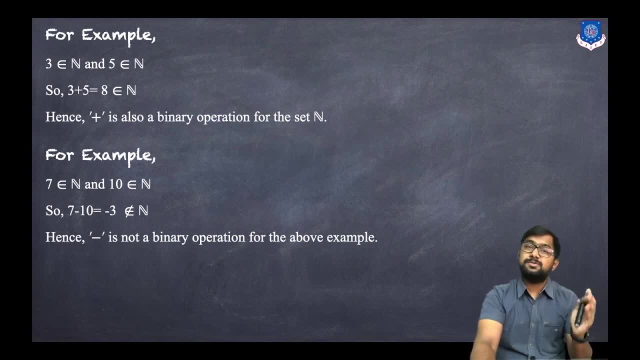 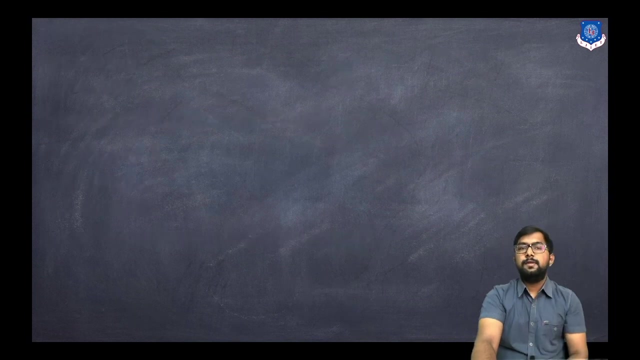 for the specific above example. Okay, Why? because the both the elements. that belongs to the set of natural numbers, but there, after applying the operation, we are getting the answer: that does not belongs to the set. Okay, So it is not a binary operation. Now what? 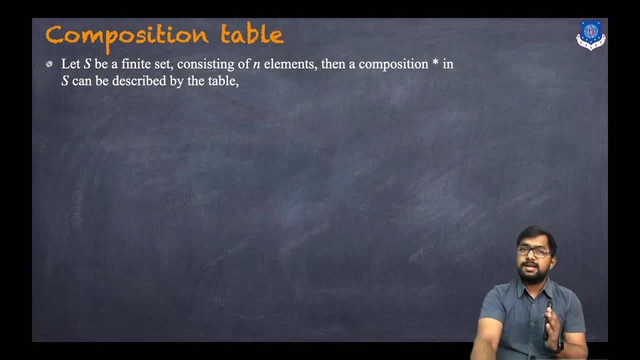 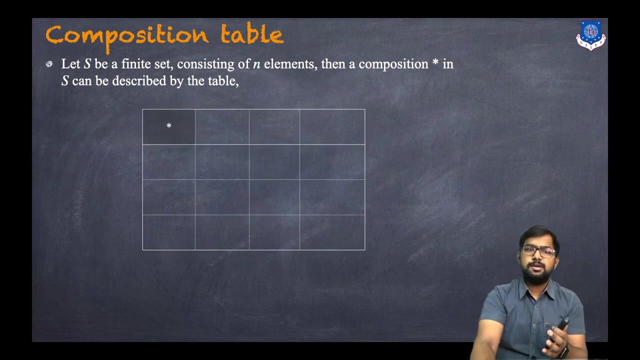 is a composition table. So let capital S be a finite set consisting of N elements. Then a composition- Here we have star In S- can be described by the table. We are taking one example. So let us consider this table. We have the star composition. Then let us 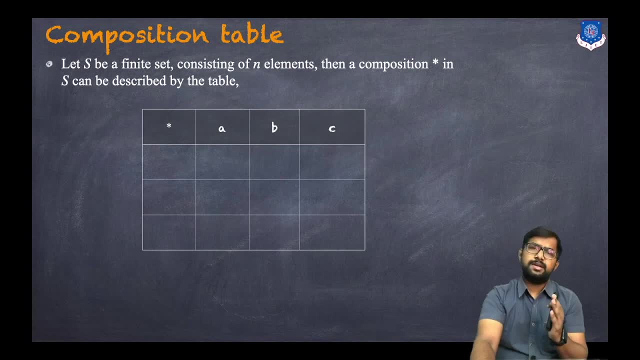 take A, then B and C. Okay, So we are taking 3 elements Now in same manner in row. we will get A, B and C. Now suppose the answer of this portion So that is A star A. So we will denote it as: 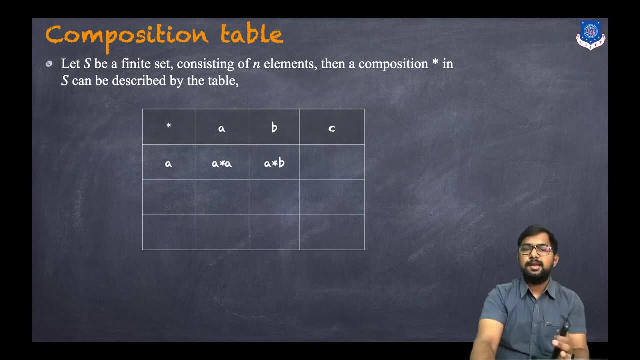 A star A, then in same manner A star B and A star C. Now in second row, here it will be B, as we have 3 elements Now. here it will be B star A, So column to row. So B star A, in same manner B star B, then B star C, and here the element is C, Now C star A, So C. 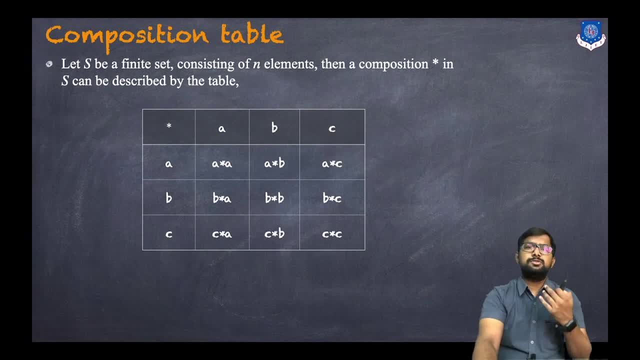 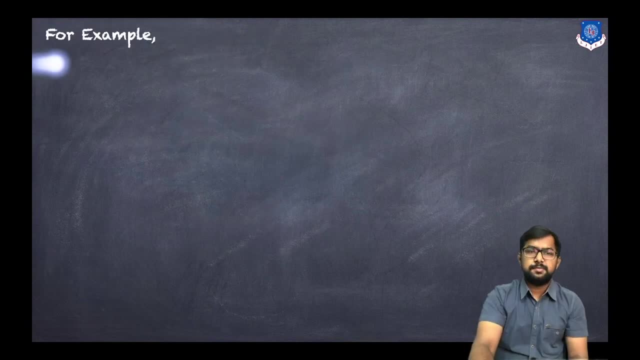 star A, C star B and C star C. So this is how we can construct a composition table. Okay, Now, for example, let us take example: So if you have the set S, 1 minus 1, I and minus I, So we have 4 elements. So how to? 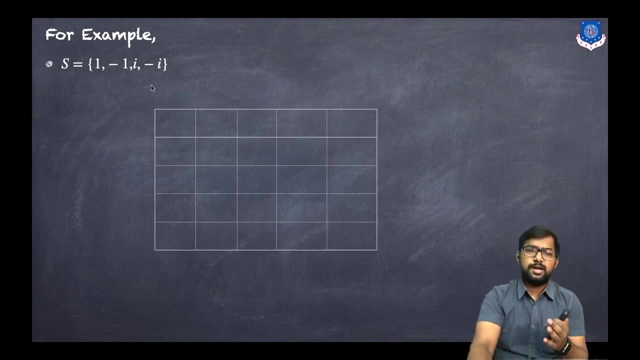 find the composition. So, as you know that here the operation is what We have taken, the operation as dot, Okay, or the product side. So in column we will have 1 minus 1, then I and minus I, now like this, okay. and in same manner, in row there will be 1 minus 1, i and minus i. so here, 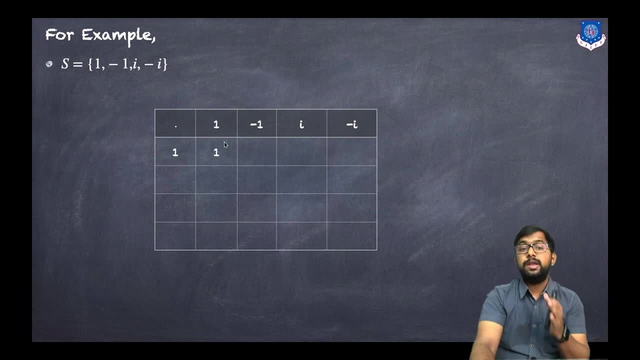 1. now what is 1 into 1? so it is 1. now 1 into minus 1, so it will be minus 1. now 1 into i, so i now 1 into minus. i so minus i. now the second element, so it's the second element is what minus? 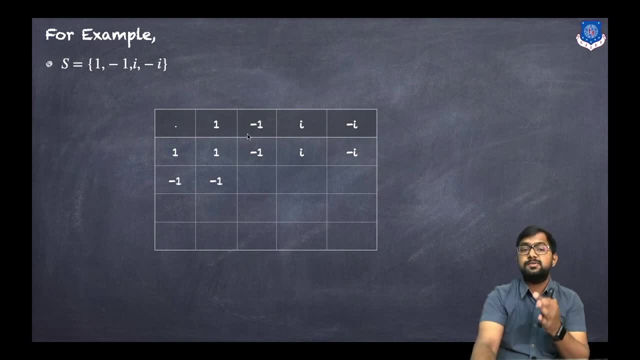 1, so minus 1, into 1. so minus 1 minus 1, into minus 1, plus 1 minus 1, i minus i, minus 1 minus i, so i now i into 1, so i then minus i, then i square. now we know that what is i square, it is. 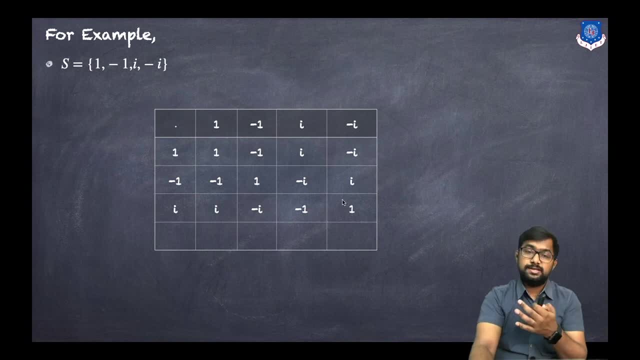 negative of 1, so minus 1. now i into minus i, so i into minus i. so minus i square right square is minus 1, so minus of minus. so that is plus 1. now minus i into 1, so minus i, minus i into minus 1. 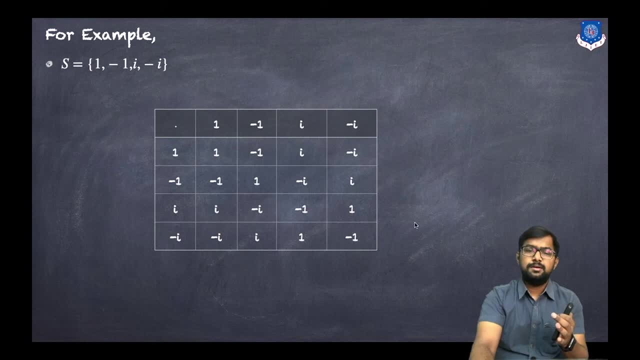 plus i, then 1 and in same manner minus 1. okay, as you can see that the all the elements belongs to the given set and the composition or the product, as you can see that the all the answers, they belongs to the given set. so it is closed under the operation this dot. 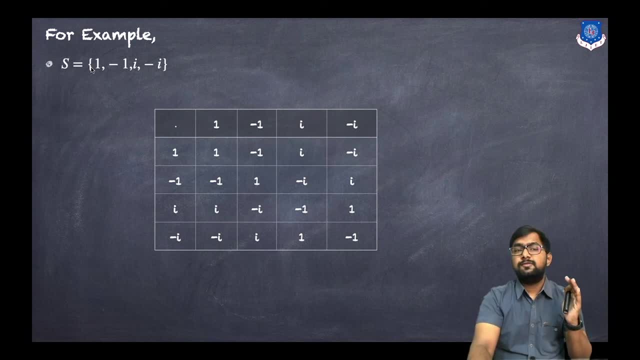 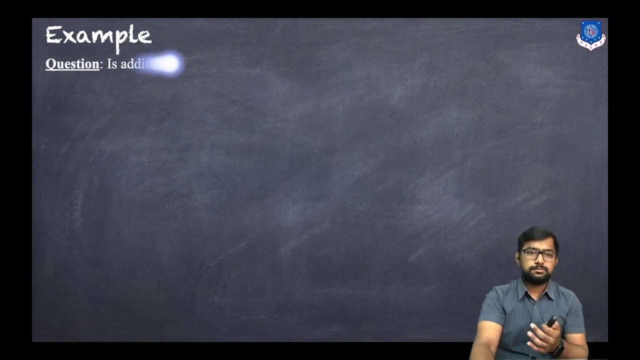 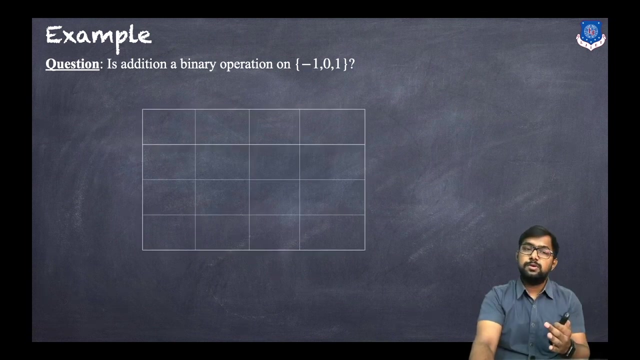 okay, so here all the answers are either from 1 minus 1 i or minus i. fine, now let us take another example. so is addition a binary operation on the given set minus 1, 0 and 1? so what we'll do will again construct a table. okay, and here we have the addition. addition is as: 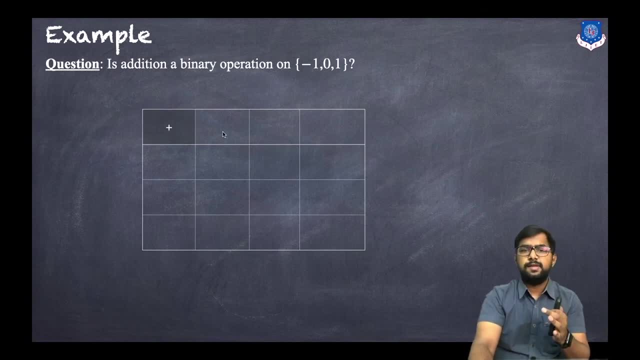 a binary operation. so we'll write idea plus, then minus 1, 0 and 1, and in same manner in droop will write minus 1, 0 and 1. okay, so minus 1. now the addition. here we have addition, so minus 1, into my sorry, minus 1, plus minus 1, so that is. 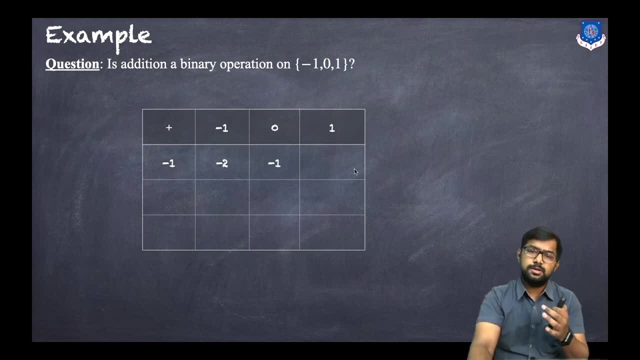 minus 2, now minus 1, plus 0 minus 1. now here it will be 0, and same manner here, 0, so minus 1, 0 and 1. right and last entry here: 1, so minus 1, then 1 and 2. as you can see that for becoming a binary operation, the closure property. 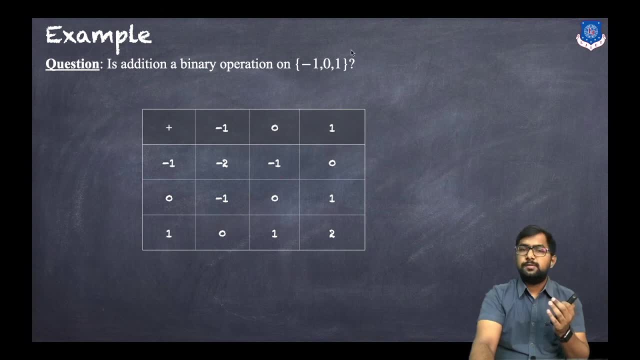 must be code. ok, so here minus 1, 0 and 1, they are the set itself. now the answers will be also from the set. but as you can see that this minus 2 does not belong to the set, Now in same manner this 2 does not belong to the set. so what we can conclude? it is not. 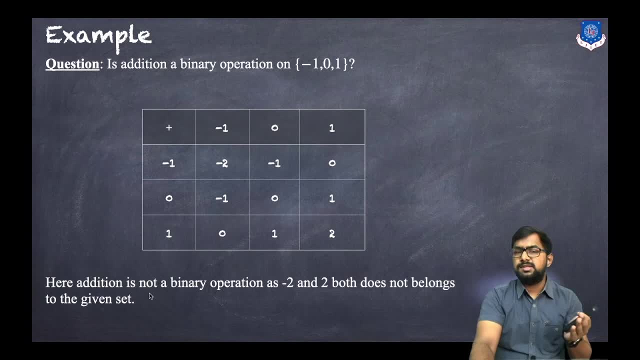 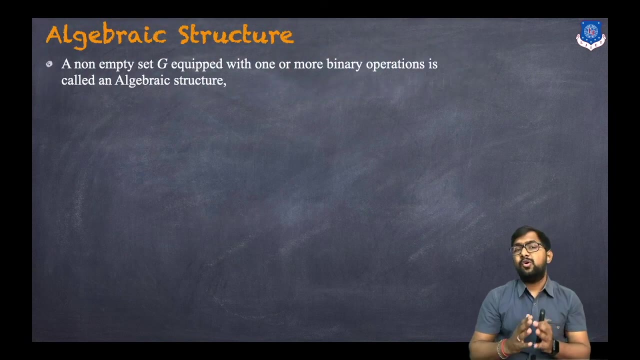 a binary operation. So yes, here addition is not a binary operation. why? because this minus 2 and 2, they both does not belong to the given set, so it is not a binary operation. Now let us discuss what is the algebraic structure. So a non empty set- let us take G- equate with one or more binary operations, is called an. 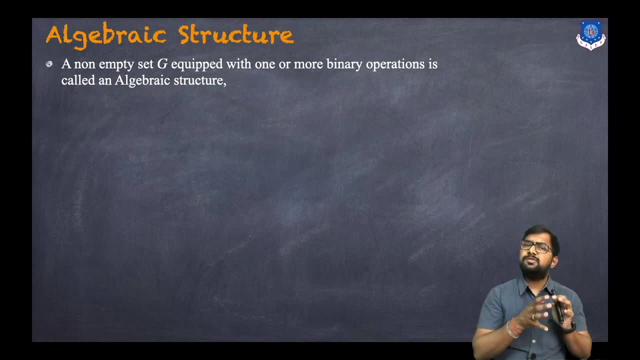 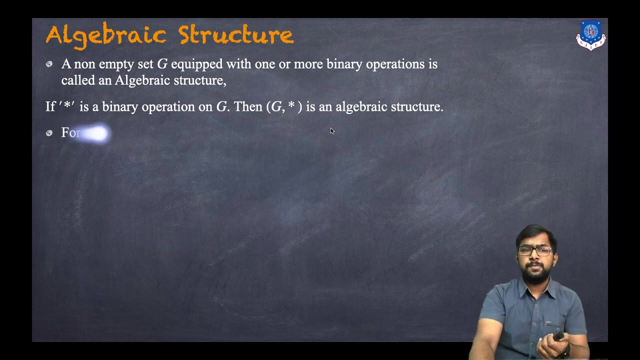 algebraic structure. So a non empty set with one or more binary operations is called algebraic structure. So now, if the star is a binary operation on G, then the set G comma star- this is the notation- is an algebraic structure. fine, Now, for example, we have this N plus it is a binary operation. 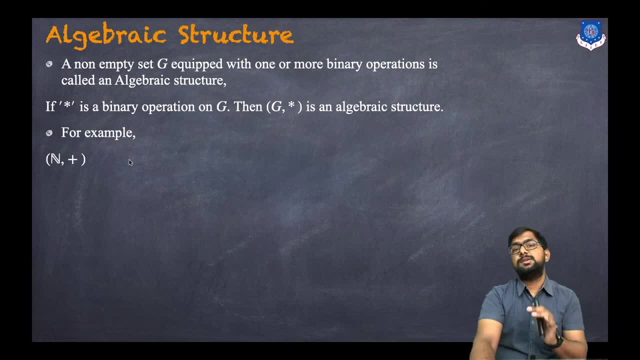 So set of all natural numbers, with the binary operation plus, it is a binary operation. Now, in same manner, we have discussed This N and minus, so that is not a binary operation. that is, we already discussed right N and minus. so set of natural numbers and the operation is minus, so it is not a binary operation. 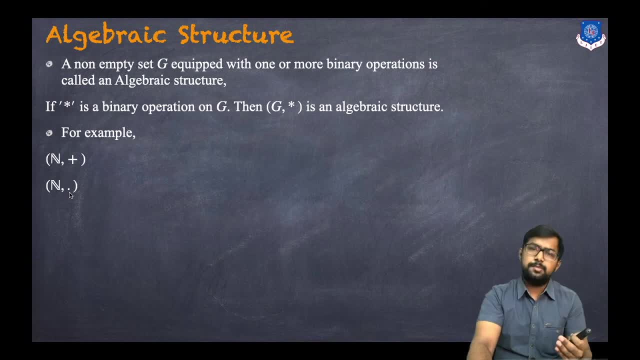 But the set of natural numbers and dot or the multiplication. that is a binary operation. So if we take any two elements and the multiplication, what we will get, so it will be, it will belongs to the set of natural numbers. Now, in same manner, I plus. 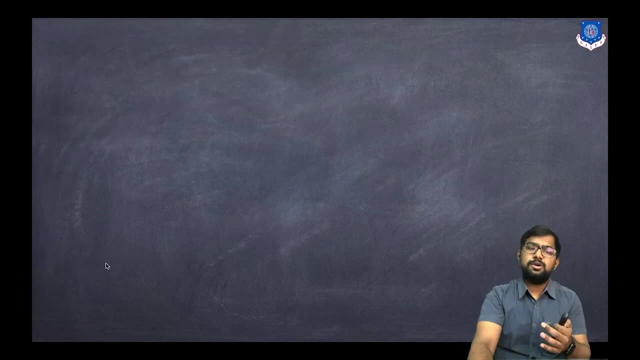 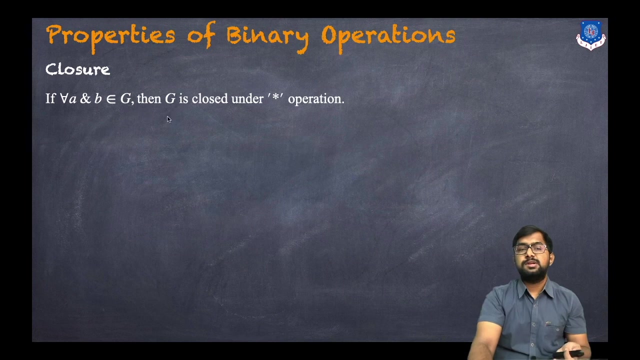 I dot set of integers, then I dot, and they all are the algebraic structures. okay, Now what are the properties of binary operations? So the first one, the closure property that we know. So for every A and B belongs to G. G is closed under the star operation. 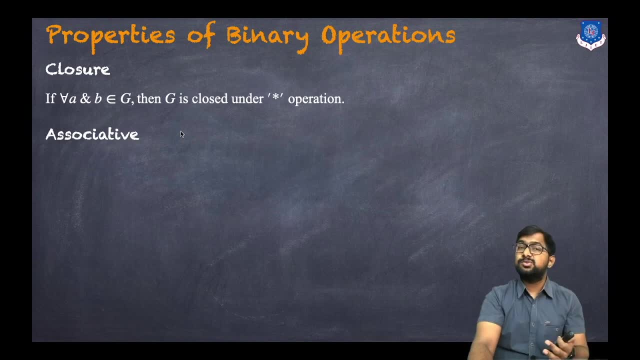 So okay, so it is a closure property. Now, what is associative property? So if we want to take three elements, So for every A B C belongs to G If this A star, B star C equals to A star B star C, So it is called associative. 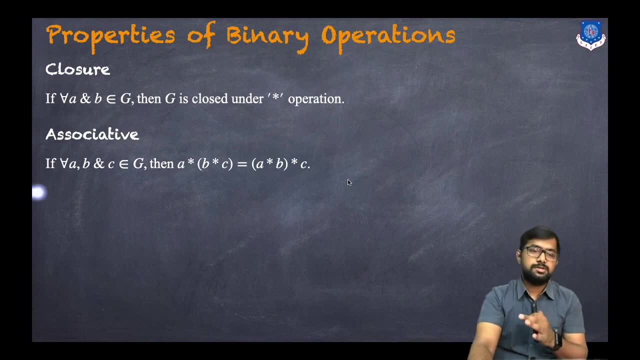 So that means we can change the brackets? the answer won't change. For example, if we take 2, 3, 5, they belongs to I. then what? this 2 plus 3 plus 5 equals to 2 plus 3 plus 5.. 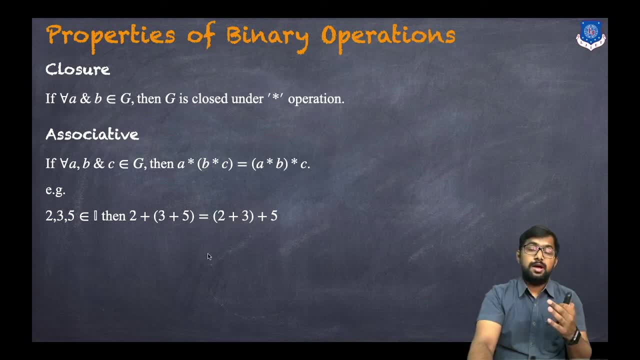 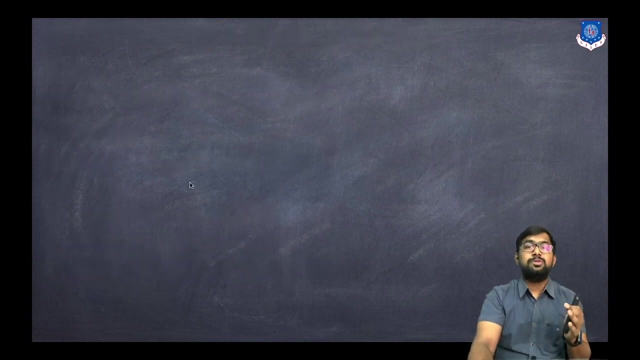 So if we change the brackets, the answer is unchanged. okay, So it is associative one. Yes, Now yes, and also for dot, or also for multiplication. it is correct and fine. Now, therefore, plus and dot, both are what they are associative. okay, Now, what is a commutative property? 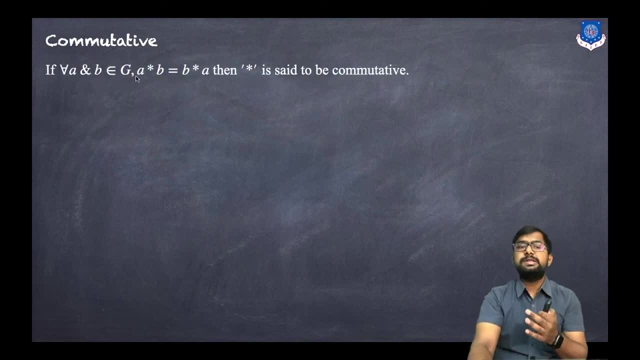 So if we have two elements for every A and B belongs to G, This A star B equals to B star A. then star is said to be a commutative, So that means we can change the order. So either we will calculate this: A star B or B star A. 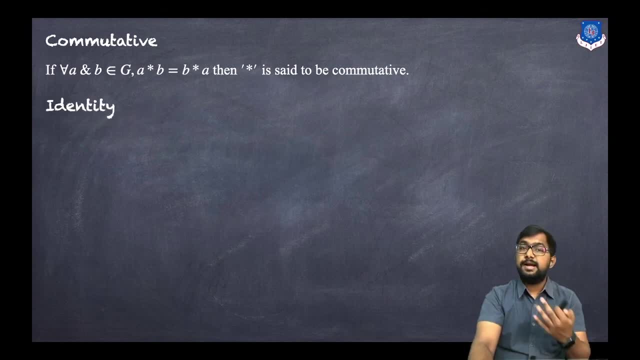 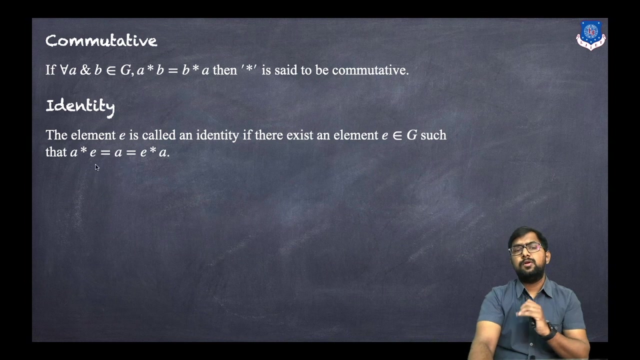 The answer won't change. Okay, Now, what is the identity? So the element E is called an identity. if there exists an element E belongs to G, the given set, such that this: A star E equals to E star A equals to A, or A star E equals to A itself equals to E star A. 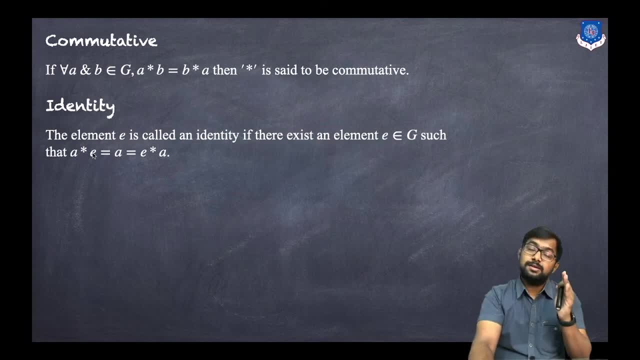 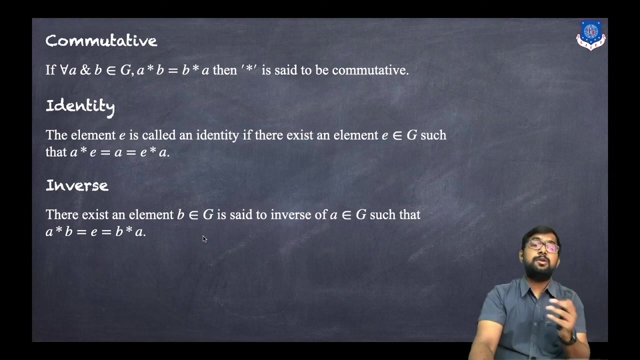 So that means they are commutative. also, and if we multiply the given element with the sum E and we will get the same element, Then it will be an identity element, Just by its name. okay, Now what is the inverse element? So there exists an element: B belongs to G. Let us say B belongs to G is said to be inverse. 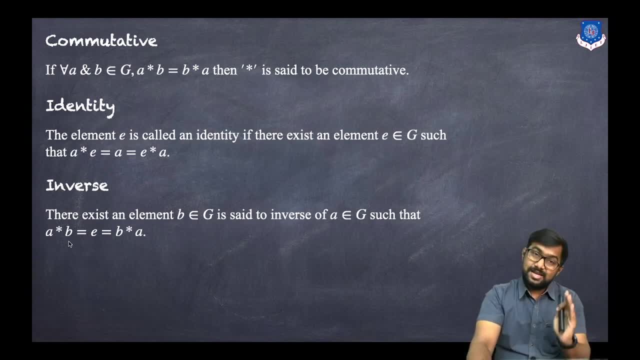 of A, such that what this A star B equals to E, equals to B star A. So that means what A star sum B and after multiplying that will get the identity element. So that is this above. So that is E and it is same as B star A. 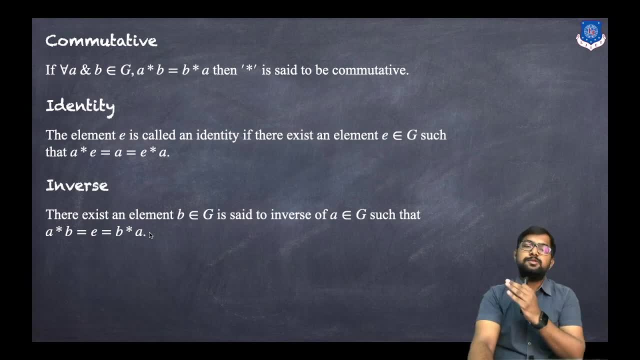 Okay, So A star B equals to E, equals to B star A. So what is the inverse? So A, into its inverse, will get the identity element. So this is the inverse. Fine, Thank you.